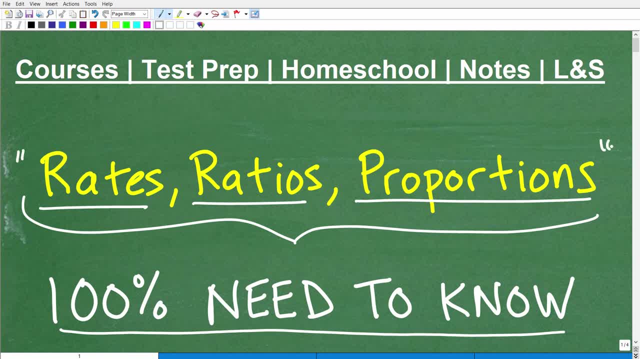 all kind of interrelated. Generally speaking, when you study this you don't study rates by themselves. You study rates and ratios and proportions. So if you know what a rate is, a ratio is and a proportion, if you have a good sense of what they are, put that into the comment. 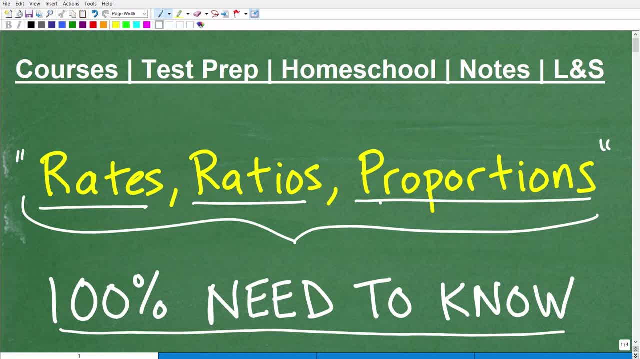 section. I'd be interested in seeing what your definitions are for these very important math terms, But I'm going to go over this here in one second so you can walk away having a great understanding of rates, ratios and proportions. But before we get going, let me quickly introduce. 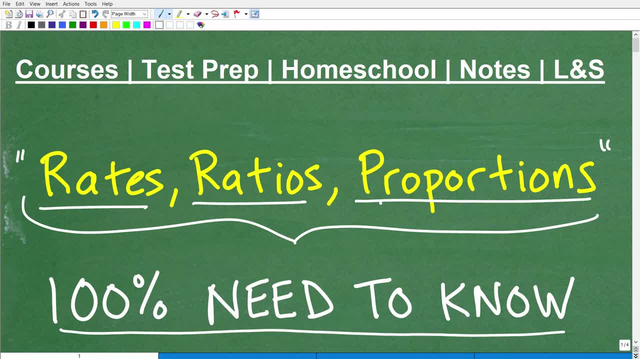 myself. My name is John. I'm the founder of TC Math Academy. I'm also a middle and high school math teacher. I've been teaching math for decades And if you're struggling in math, please do not give up. There is absolute hope for you. But the main thing you need is great math instruction. 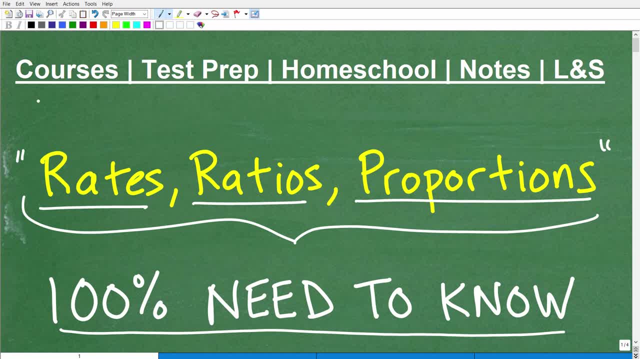 clear, understandable and comprehensive, And that's where I can help you out. So if you're at the middle school, high school or even college level in terms of mathematics, check out my math in the description of this video. I promise you'll like what you will see Now, if you happen to be. 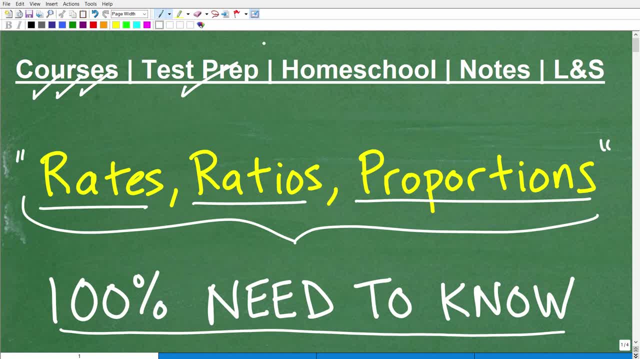 preparing for some sort of test with the math section. there's a ton of them out there, Things like the SAT, ACT, ASVAB, maybe the GED or a teacher certification exam. I have a ton of test prep courses that you might want to check out. If you homeschool, I have award-winning homeschool. 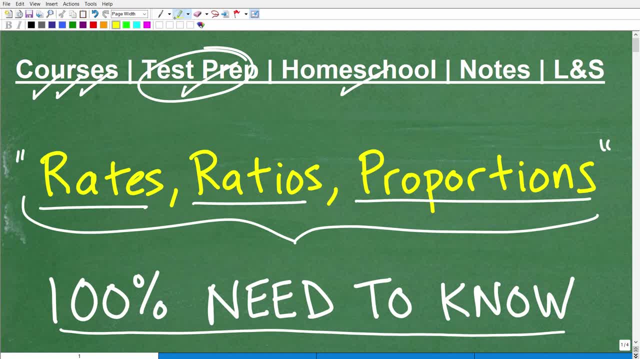 math courses for middle and high school mathematics, something you might want to check out. And if you need a pair of math notes, hopefully you have your own. Okay, great math notes is so critical to your success in mathematics. But if you don't have a pair of 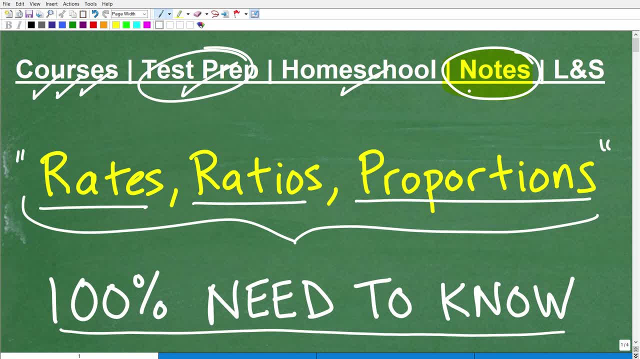 great math notes. you can check out mine. I'm going to leave links to my notes in the description of this video And if this video helps you out, don't forget to like and subscribe, as it definitely helps me out. But let's go ahead and get into rates, ratios and proportions And we'll start. 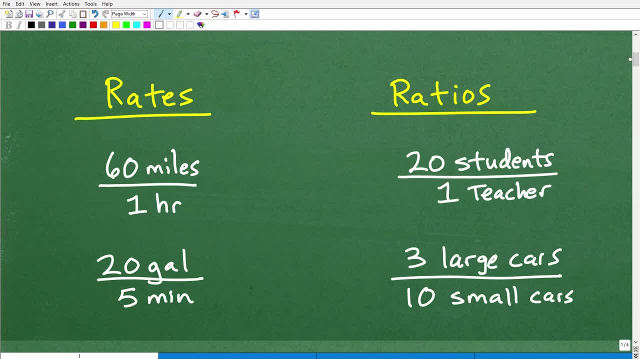 off with rates and ratios. So, what is a rate? What is a ratio? Well, effectively, I just want you to: these are essentially fractions. okay, They are fractions. So if you answered, hey, a rate and a ratio is a fraction, well, you would be pretty much correct. However, there's a little bit of a 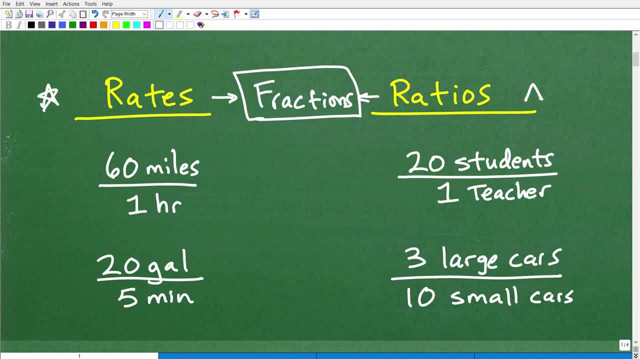 twist. okay, So we have to discuss something called the units of measure. okay, So rates and ratios are measuring something very specific, ie a fraction might be like, say, the fraction of a number. So what is a ratio? Well, this is just a fraction. It doesn't really, you know, we 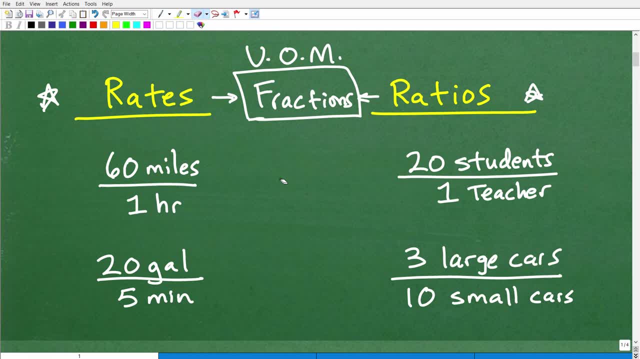 wouldn't say that this is a rate or a ratio, because what makes a rate or a ratio is the following: So let's go ahead and talk about rates here Now. a rate, again, is a fraction, But what makes a rate a rate is we have to have units of measure. In other words, we're counting something. 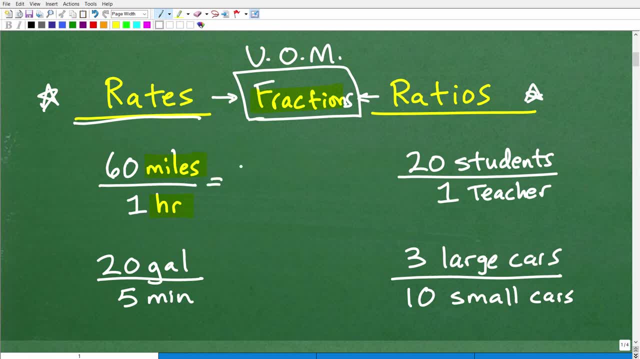 specific. So if we look at the numerator, okay, of course, a fraction, you have a numerator and a. The deal with a rate is the following: The units of measure are different. okay, This unit of measure here, okay, is completely different than this unit of measure down there. Now, what do I mean by unit? 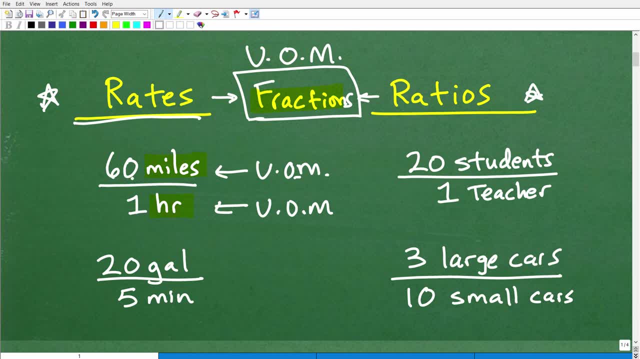 of measure. Well, here I have the fraction 60 over 1,. okay, So it's just 60,, but it's 60 over 1.. What am I counting up here in the numerators? Well, I'm counting miles. What concept is this? 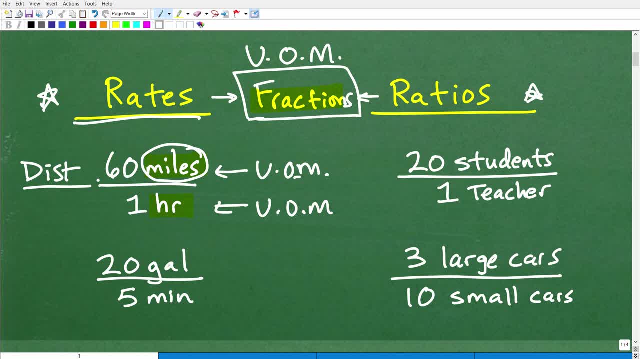 Well, that's distance, right. So 60 miles is a. the units of measure is, of course, miles. But what am I measuring? Well, I'm measuring distance, And let's take a look down here in the denominator. We have one hour. okay, What's the unit of measure? 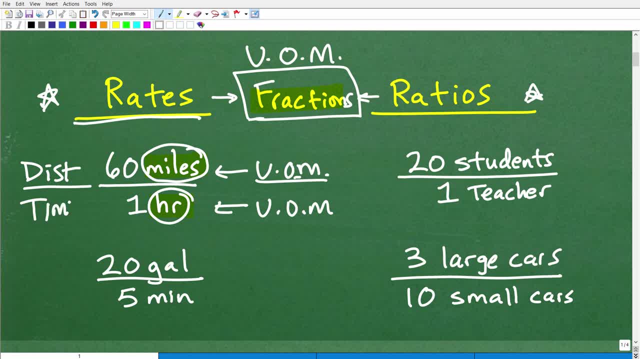 Well, it's hours, but I'm basically counting time. So you're comparing two different units of measure. So technically, that would be the technical definition of a rate. You're comparing two different units of measure, so ie distance versus time, And it could be two completely. 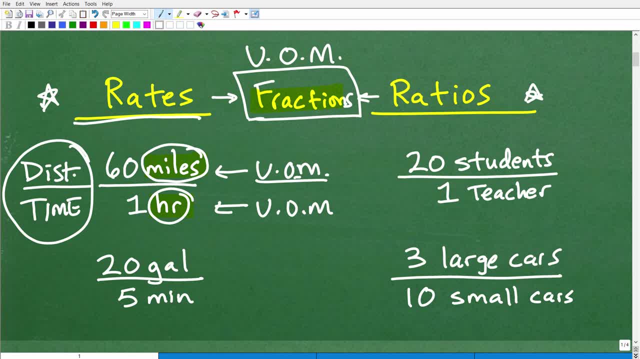 um other type of units of measure. It doesn't have to be just distance and time, like something like here: 60 miles per hour. okay, So we have 60 miles And, by the way, the fraction bar in a rate. 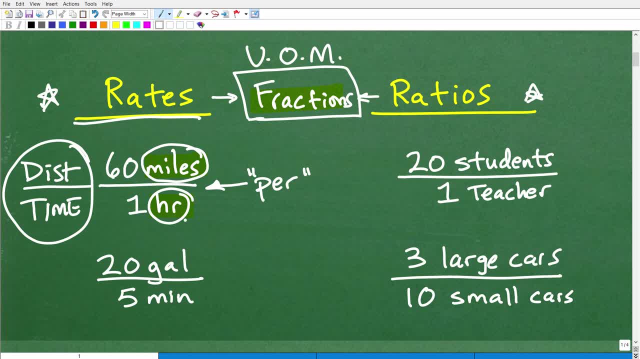 you say the word per okay, So 60 miles per one hour, Of course you would write this as 60 miles per hour. So anytime you hear that word per okay, we're talking generally about a rate. All right, let's take a look at another example of a rate. 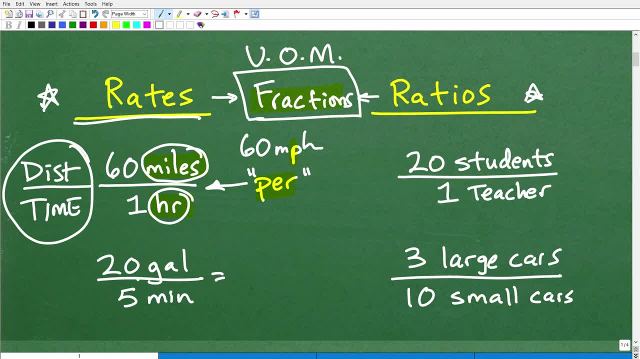 So let's say you have a pump that can pump out 20 gallons out of let's say you know a pool of water or whatnot, every five minutes. okay, This is the rate of the pump. So you know. 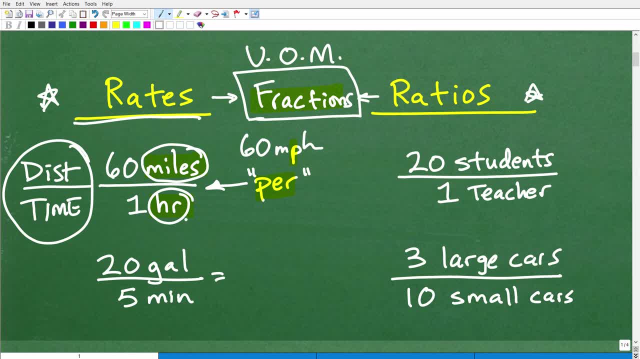 what's the rate of a car, for example? Well, it might be 60 miles per hour. What's the rate of a pump? Well, it's 20 gallons per five minutes. So this term rate often gets associated with the concept of like speed or velocity. okay, How fast something goes. 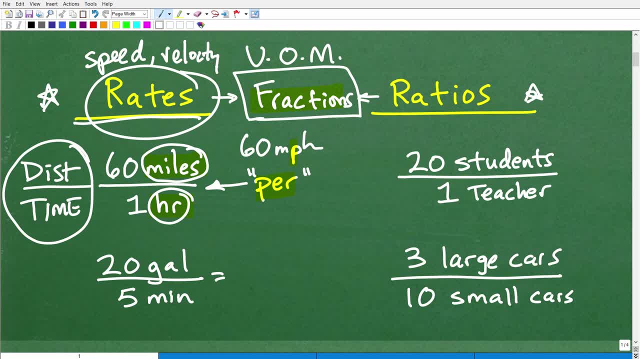 So, hey, you know what's the rate of a vehicle, etc. etc. So you might have, you know, kind of a pretty good idea that that's how this word is used. But let's go over here and continue to take a look. 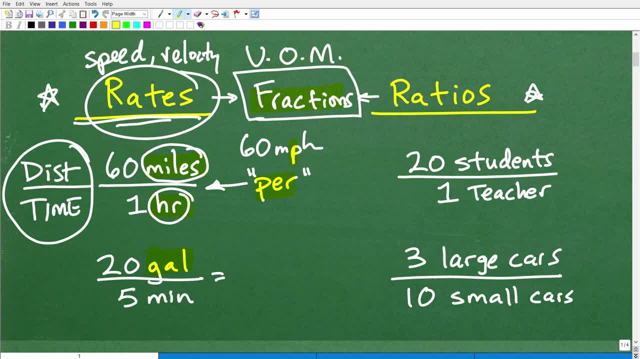 at this second example of a rate. So what am I comparing here? Gallons, okay. Well, this unit of measure here, gallons, is completely different than this unit of measure down here, which is minutes. So gallons is a measurement of volume and minutes is, of course, time. So again we're. 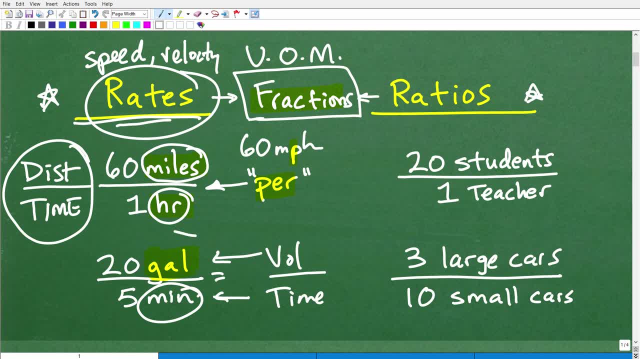 making a comparison. We have two completely different units of measure and expressed as some sort of fraction, That is a rate. okay, All right. So now let's take a look at ratios. So ratio is basically the same kind of concept. okay, as a rate, We're comparing units of measure. However, the units of measure here. 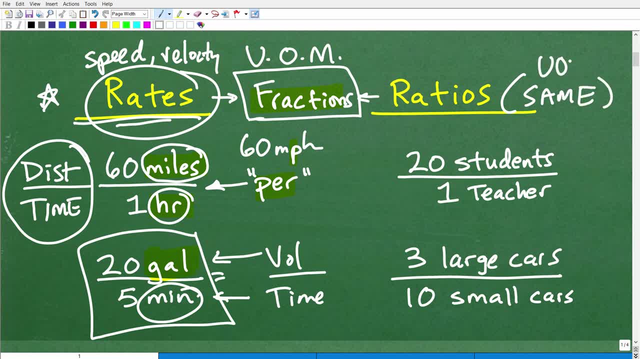 are the same. okay, So effectively, unit of measure is the same. Let's go ahead and make some nice little, lovely little notes here for you And over here. units of measure are different. okay, We're comparing two different units of measure Here. 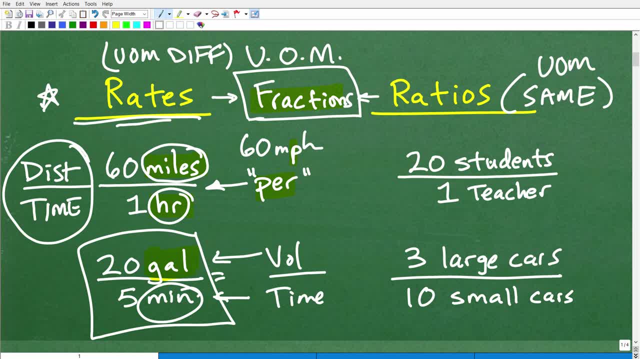 we're generally- well, not generally- we are in fact counting the same units of measure. There's a little bit of a twist here. So let's take a look at an example of ratios, because students get confused with this. So a typical unit of measure, you might, or ratio, you might, have heard. 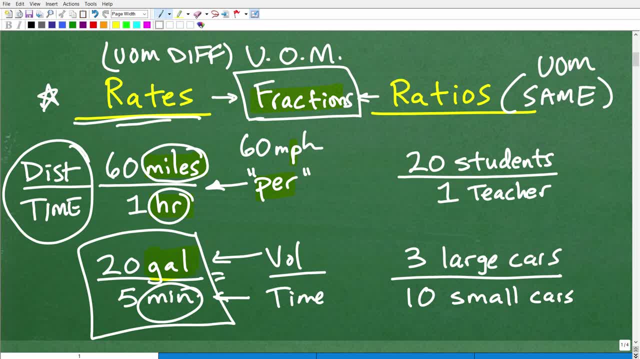 is like a student-teacher ratio. So, for example, let me have a look at this, So let's take a look at this and actually erase this here a bit and give ourselves some room. So a student-teacher ratio is: here is the classroom, here is the teacher and here are the students. So, typically, what schools? 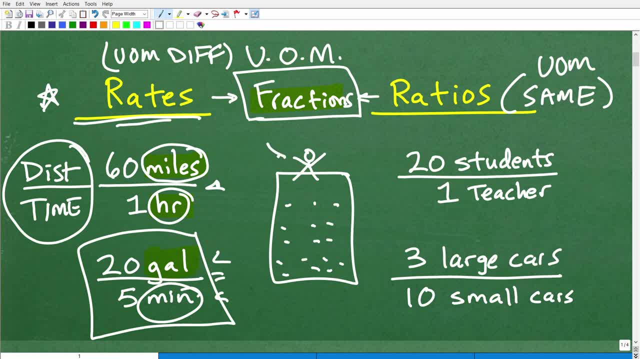 or colleges like to you know, advertise is: hey, we have one teacher per this many students. That's called a student-to-teacher ratio. So here's an example of one. So for every 20 students, you will have one teacher, okay, or one teacher per. 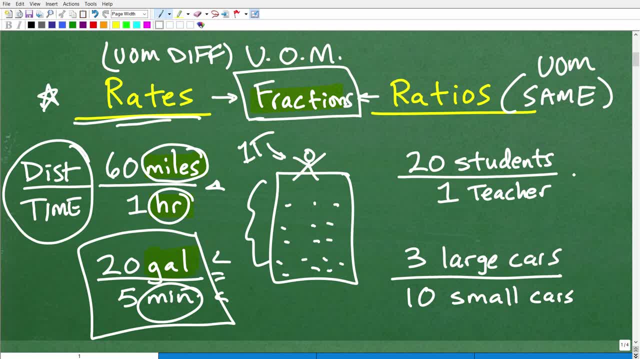 two every 20 students. So in ratios the fraction bar right here is expressed with this word two. Unlike over here, when we're dealing with rates we have like 60 miles per one hour, Here we have 20 students, two one teacher or one teacher. two every 20 students. So the word two is associated. 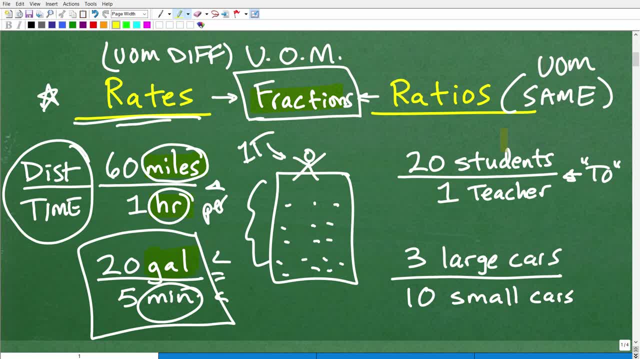 with ratios, But let's get back to the main definition. Here we're saying: well, this is what we're counting, teachers, The units of measure are different. No, they're not different. okay, What we're counting are people, human beings, right? So 20 people which we named these people? 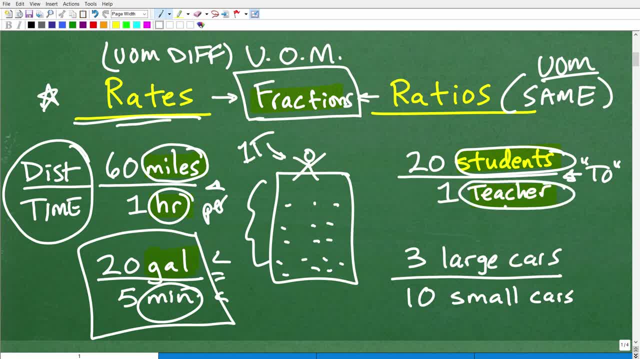 students. and then this person here is a teacher. Now, some of you might say: well, a teacher is not a human being. Ha ha ha, That's a little joke. But yes, indeed, we are all part of the human race. 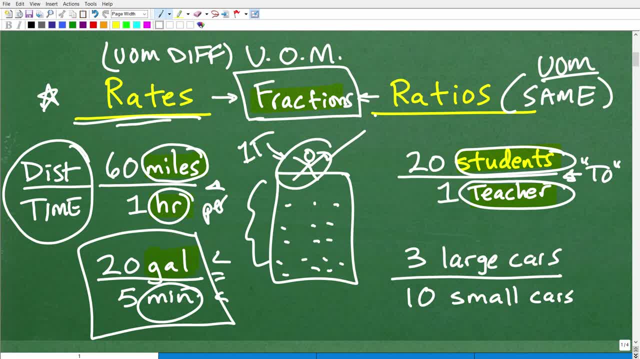 students and teachers, especially math teachers. right, But anyways, so you get the idea. So don't you hear? okay, You're still counting the same thing conceptually. So that is a ratio. Let's take a look at another example of a ratio. Let's say: in a parking lot you're counting all the 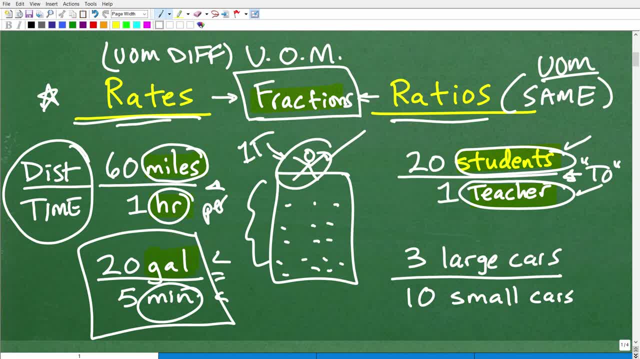 cars and you notice, for every three large cars you have 10 small cars. So this is a ratio to maybe large to small cars in a parking lot. So again, you're using the word ratio. You wouldn't say the rate of large to small cars in a parking lot. That's incorrect, right. 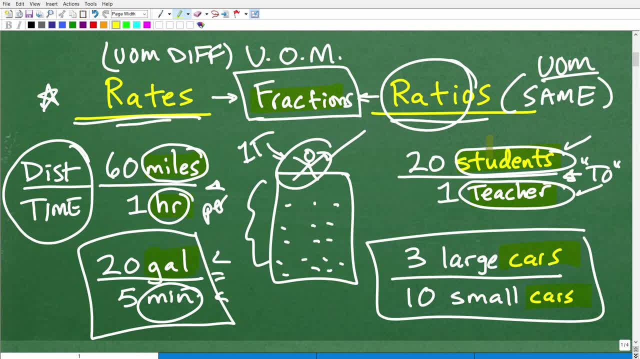 Because here we are comparing cars to cars- Okay Here. people to people were here. It's completely different distance to time or volume to time, Okay, All right. So rates and ratios are fractions, but we have to be very specific about the difference here in terms of units of measure. 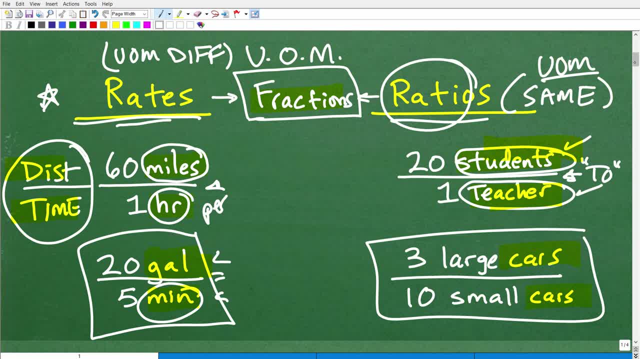 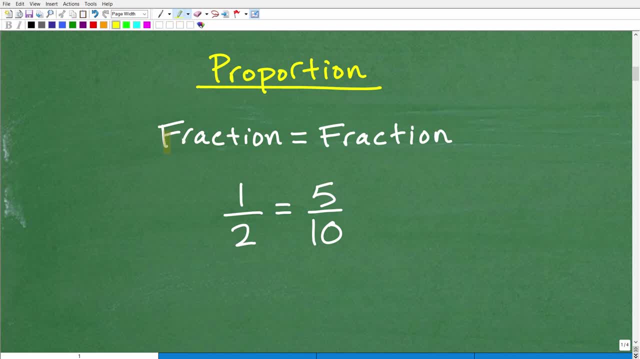 All right, So hopefully this has cleared up any confusion, and now let's move on to proportions. Okay, So what is a proportion? Well, it's very, very easy. A proportion is simply one fraction that's equal to another fraction. So here I have one fraction, one half. 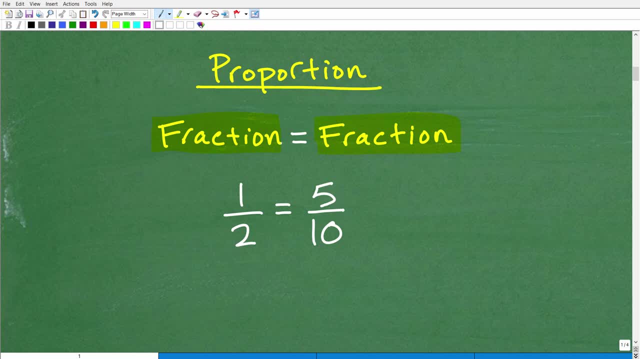 and here it's equal to the other. this fraction here- five tenths, Now one half, could be equal to all sorts of fractions. three, six, I can make all sorts of comparisons. Four over eight is equal to 50 over 100. So all these right here would be considered proportions. So anytime you 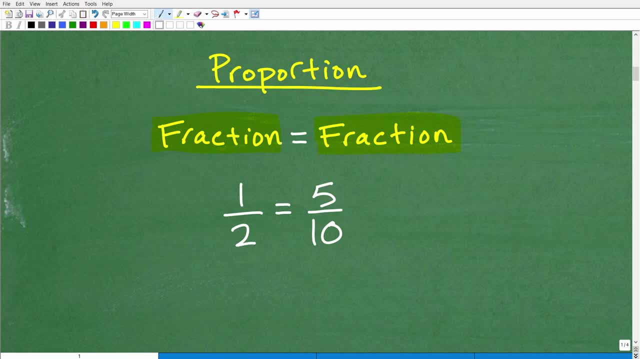 have two equal fractions, you have a proportion. So the main thing you need to know about proportions is there is a property called the cross product. Okay, The cross product super, super important And basically the cross product is this: Okay. 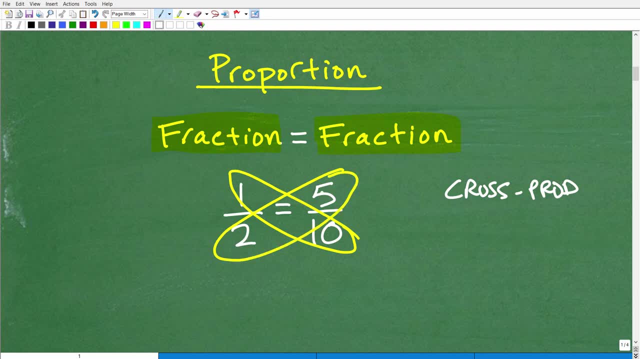 If we multiply crosswise. so let's go here: two times five. two times five, that's going to be equal to this cross product right here, one times 10.. So two times five is 10,, one times 10, of. 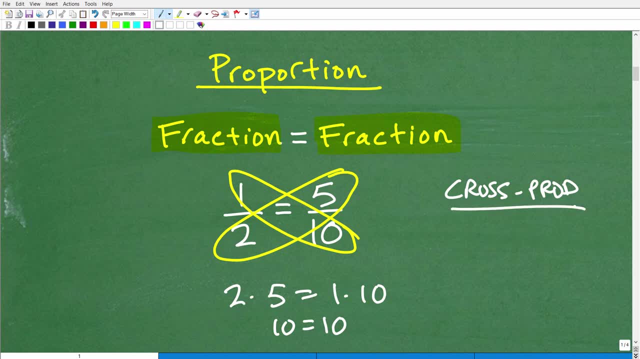 course, is 10.. So, when it comes to a proportion, it's going to be equal to the cross product. the cross product, is true, And this is the main thing that we use to solve proportion problems. So you might be asking yourself: okay, we're talking about, you know, one fraction equal. 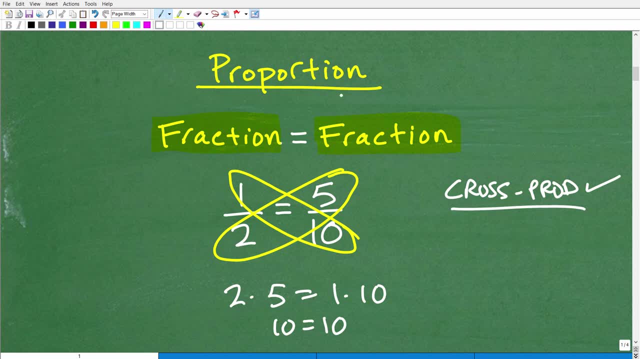 to another fraction. So how does proportions relate to rates and ratios? Well, rates and ratios are fractions, Okay, So when we're dealing with rates and or ratio problems like these, of course it can be expressed as fractions, So we can oftentimes set up a nice proportion to solve. 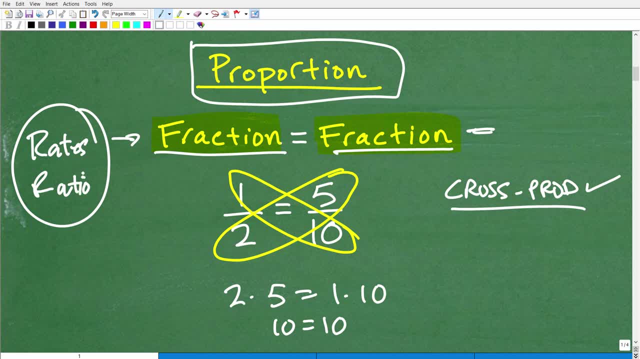 these problems. Okay, Basically, this is how you solve rate and ratio problems- is through this concept of setting up a proportion, because you know a rate and a ratio is a fraction. So we can set up two equal fractions or two equal ratios or two equal rates. then we can solve these problems. 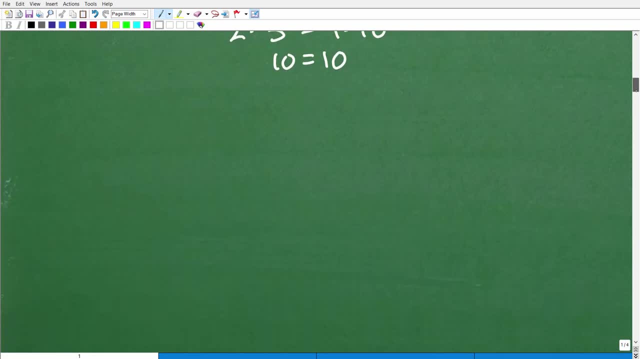 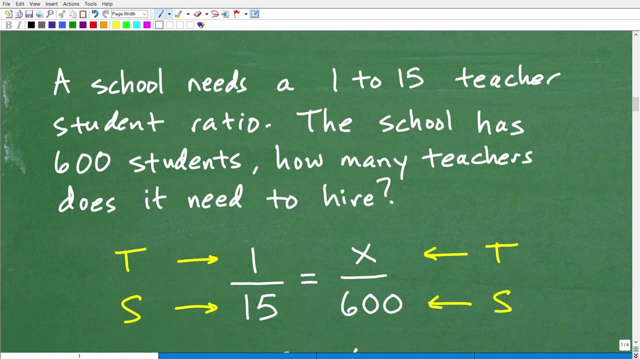 using the cross product. So let's go and take a look at one quick example. All right, So rates, ratio and proportion. so this is a basic example, So let's go ahead and read it. So it says a school needs a one to 15. 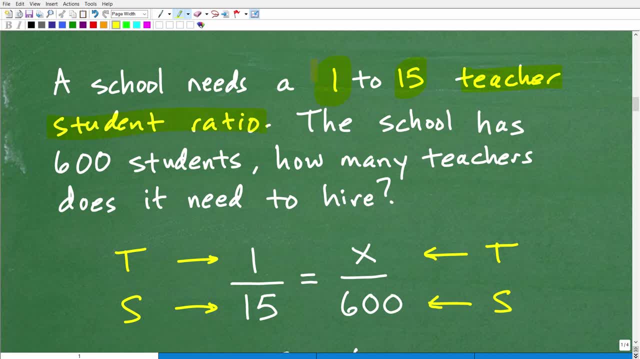 teacher student ratio. ie for every 15 students there can only be one teacher. Okay, So the school has 600 students. How many teachers does it need to hire? So a lot of you could probably reason this through. you know, even if you didn't understand ratios, proportions etc. 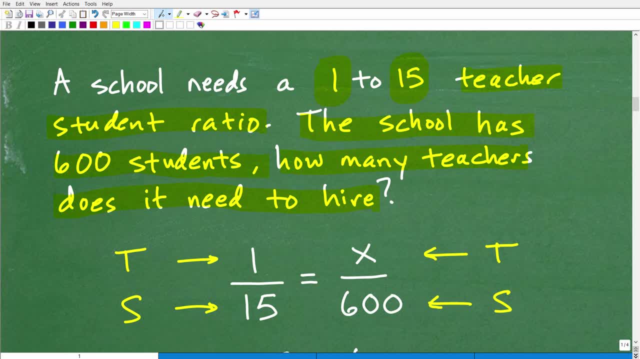 You probably kind of figured this out, But let's go ahead and set this up. So the way you want to set up a problem like this is one recognize that you're dealing with a ratio. Okay, So a school needs a one to 15 student teacher ratio, right, One to 15.. So anytime you see something like this, 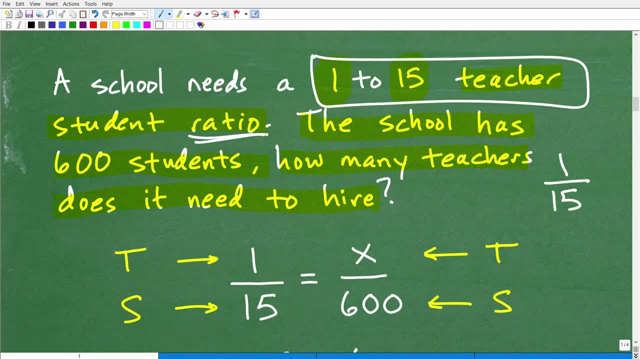 one to 15, you can express that as one to 15.. We talked about that right, That this little fraction bar is the word two, So one to 15.. This is a ratio, So let's go ahead and set this up. 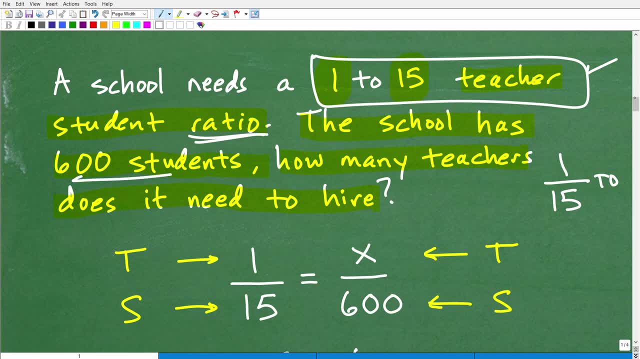 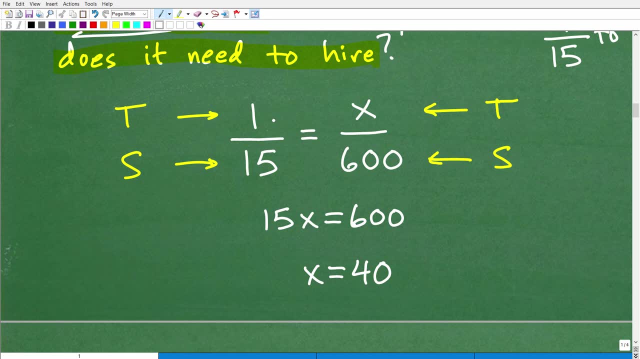 Now we have to use the rest of this information, And the idea here is to set up a proportion. So let's go ahead and take a look at this kind of the technique you use. So the first thing is you write down the ratio that you're given in a problem. Okay, So this is a very typical basic. 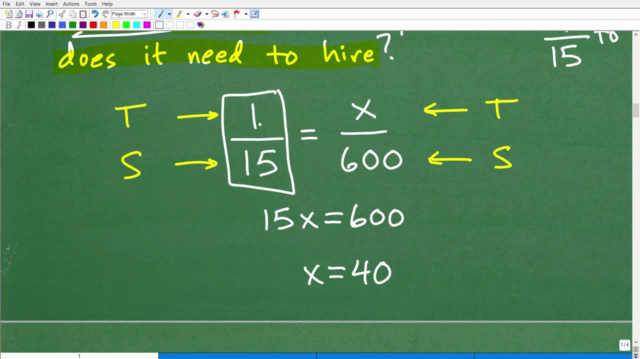 type of rate, ratio and proportion type of problem. So we know that we have one teacher to 15 students as a ratio. Now just write that down And then you're going to have a ratio. You're going to have a ratio down right here, but you have to be very, very mindful of what the 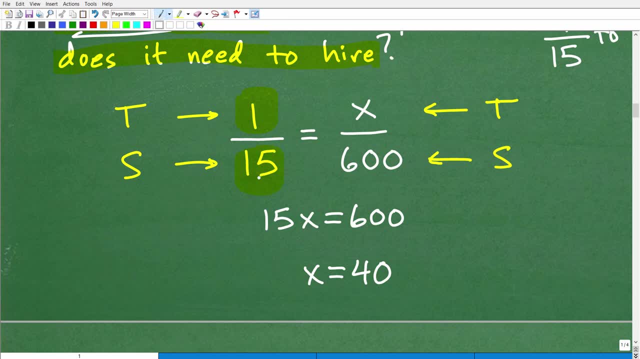 numerator and denominator are measuring. So one to 15, the numerator is measuring the teachers and the denominator is measuring the students. So we want to do is figure out how many teachers write for 600 students. So you want to construct another fraction. Remember, we want to set up a. 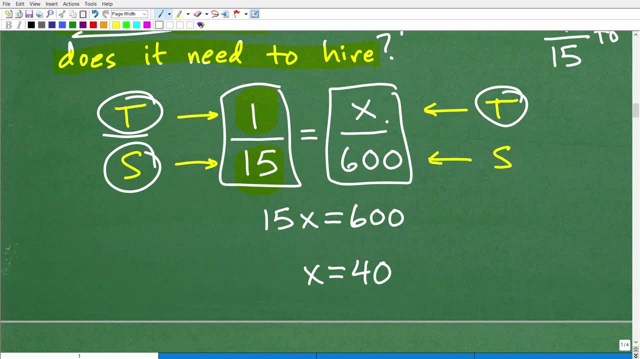 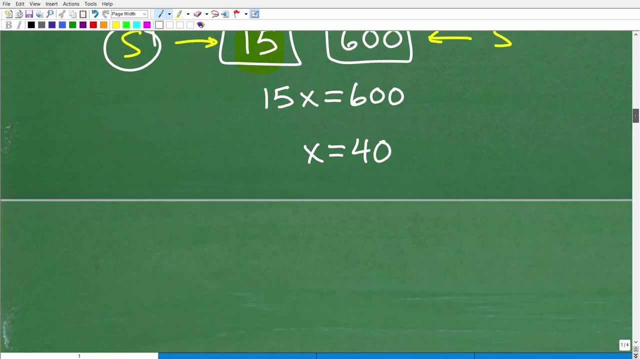 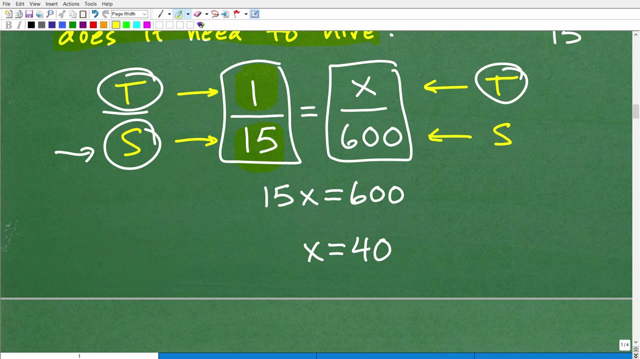 proportion. That's the main idea here. So we have one ratio equal to another ratio And what the information we have is that we have 600 students, So one to 15, right here. well, we have the student information, That's 15.. That's the denominator. So we're going to put 600 here as 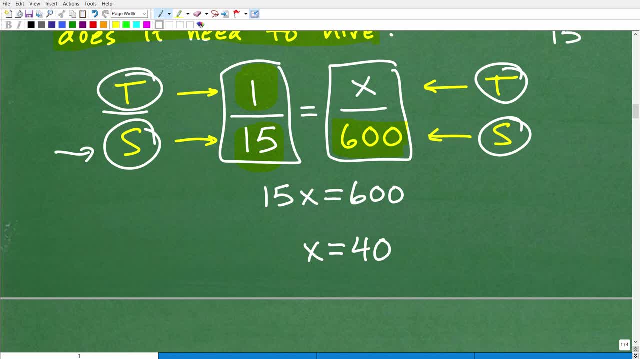 our students. Okay, So this is a common error, commonplace where students get confused. They'll set up a ratio or they'll set their proportions incorrectly. Just remember that over here we have teachers to students. So on the right-hand side, 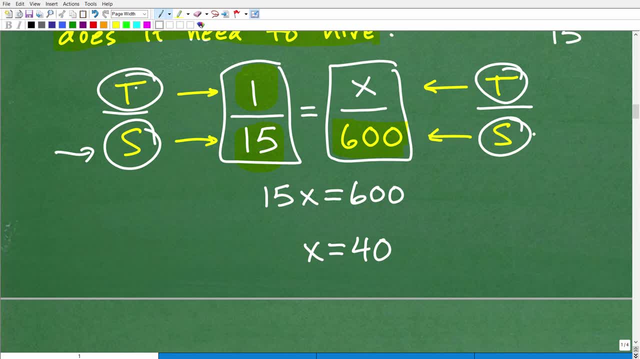 when you're setting up this fraction, you have to have the units of measure in the same consistent place. So students are down in the denominator, So we have to put students in the denominator on here. So we have 600 students, but we don't know how many teachers. That's what we're trying to. 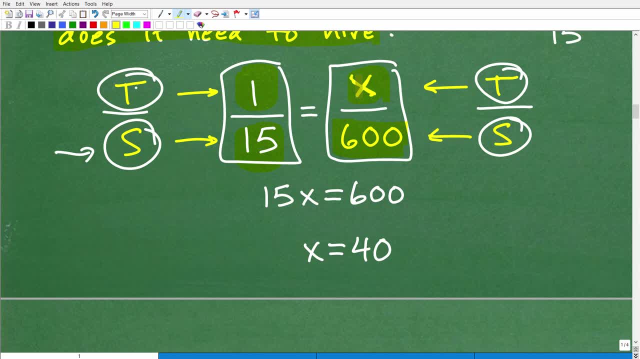 look for. So this is the variable we're trying to solve for. Okay, All right. So this is how you set up a proportion. So let me go ahead and erase this. So how are we going to solve this? Well, we're going to use the cross product. Okay, This is a proportion. We're missing this value. 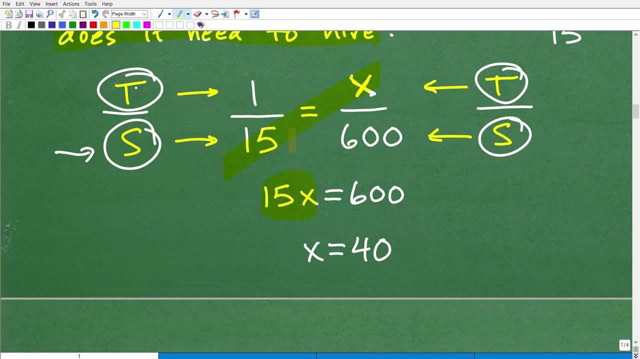 So we can go this times this. So 15 times X is 15. X is equal to one times 600. Of course, that's 600.. Now to solve for this basic equation, I simply have to divide the equation both sides. 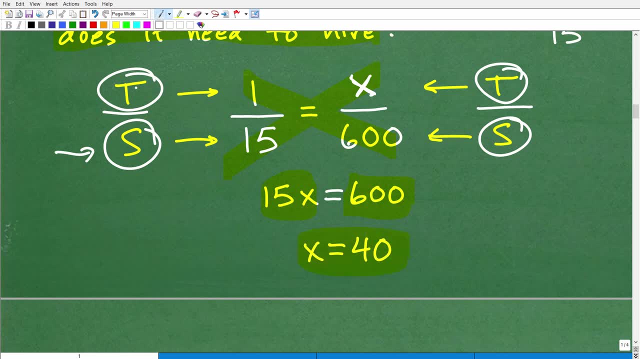 by 15 and I get X is equal to 40. So what is X? Well, that is the number of teachers needed. So you need 40 teachers, Okay, For this school size of 600 to have a consistent one to 15 student. 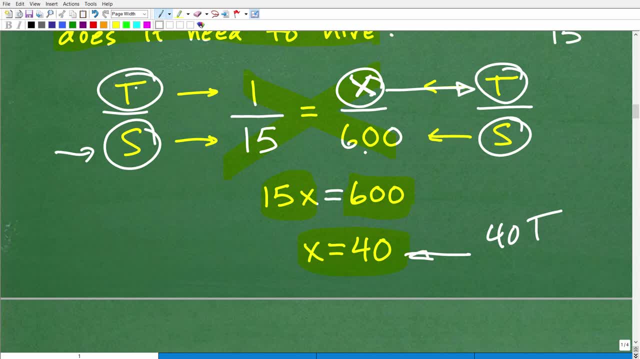 your ratio, Okay. So how are you doing with all this topic? If you knew all this stuff- and you're like I already knew all of this- I could have just skipped this video and watch something cooler. You know well, listen. you know I always try to help you, but if you know all this, 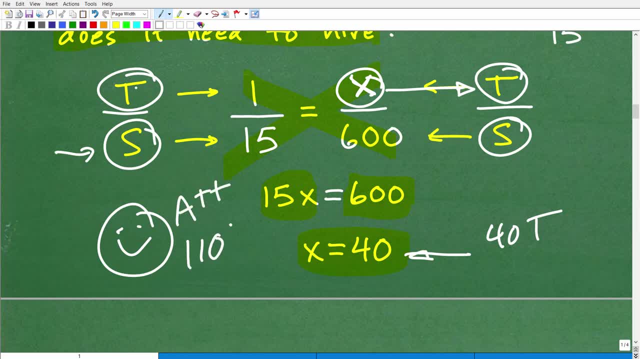 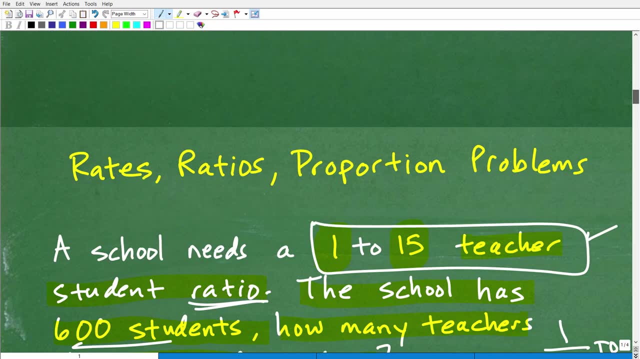 I must reward you with a nice eight plus plus a 110% and multiple stars for being such an awesome math teacher. But I suspect, uh, the majority of you, uh, you out there probably picked up on some piece of knowledge that maybe you were missing about rates and ratios. 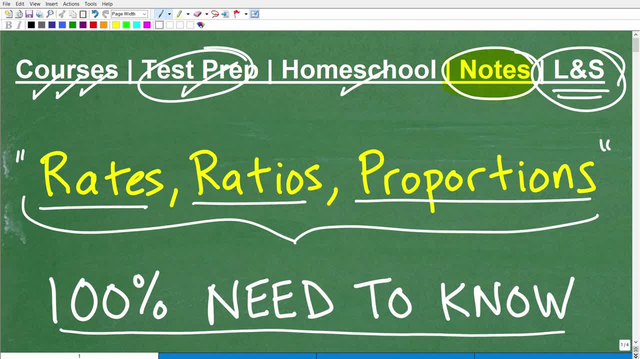 and uh, proportions, Um and again. the thing is this: you want to continue to strengthen your skills, Even if you know. you know, like a, some basics, uh, concepts about rates and a ratio and proportion. what you want to do is master this stuff. Okay, That's the key to being successful. 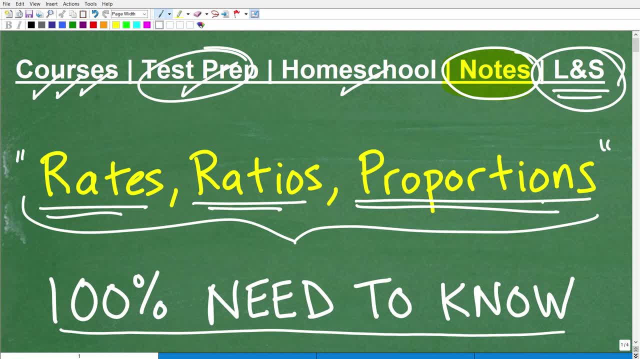 in mathematics, Don't try to learn the minimum amount. that is completely the wrong approach to learn math. You want to learn the maximum amount? Okay, So study it and, just you know, tell yourself that you can learn this stuff, because you absolutely can. 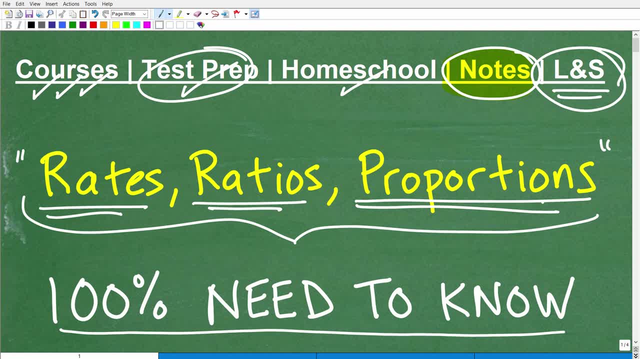 If you need more help with rates, ratios and proportions. um, also just a couple of courses in my math help program. Um, probably, uh, my pre-algebra and algebra one courses are going to be the most appropriate for those of you out there. cover both, of course. uh, uh, these topics in both. 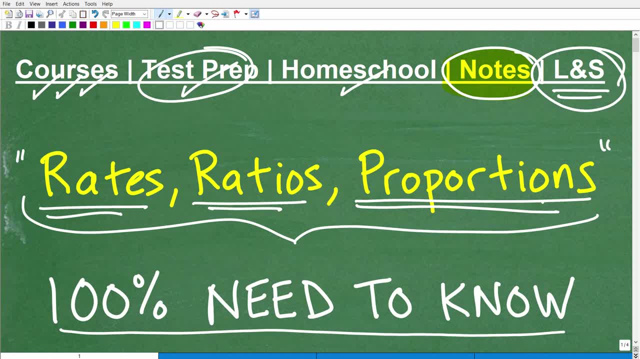 of those courses. So that's a good. that's probably my best recommendation for you. Also, I've done additional videos on my YouTube channel. You could sort through um, cause I have over a thousand plus math videos on my channel, from basic math to calculus, So you can just kind of go. 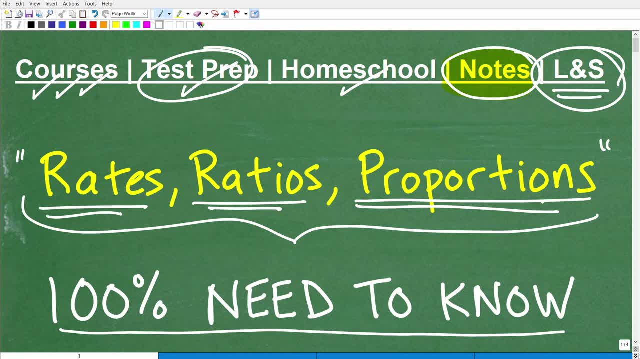 through there. I have a ton of help And, of course, I make all of this with the uh idea that I am helping you with mathematics Cause I don't want you to give up And if this video helps you out, please, uh, hit that like button and subscribe. And, with that being said, I definitely wish you 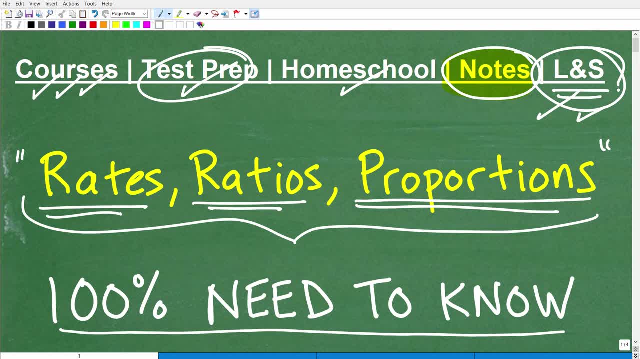 all the best in your mathematics adventures. Thank you for your time and have a great day.